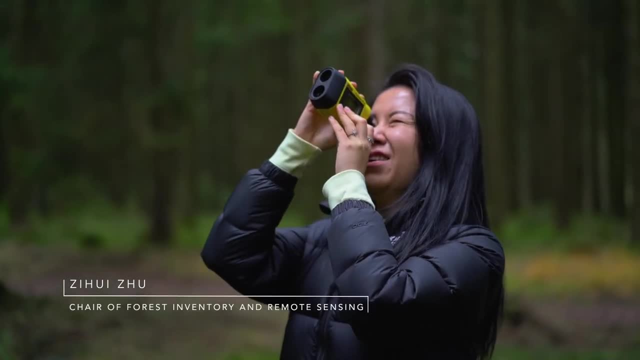 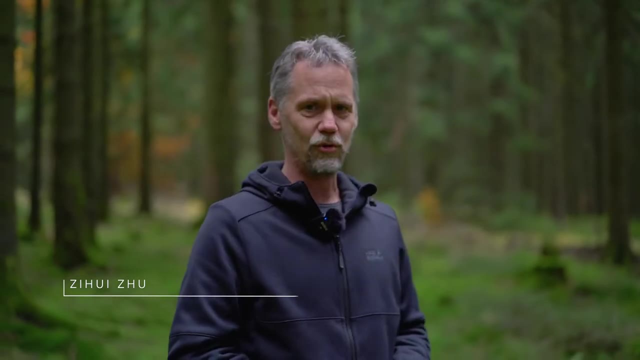 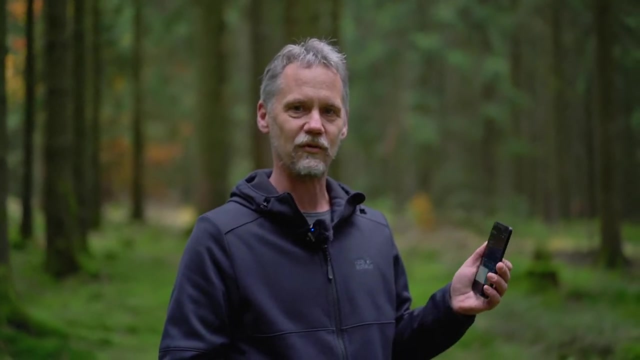 rangefinder, The tree height is 28.8.. Ok, thank you Chu. So the tree height is 28.8 meters for this spruce tree. Before I start to calculate following the formula of Denzin, we may ask our colleagues about a rough estimate. 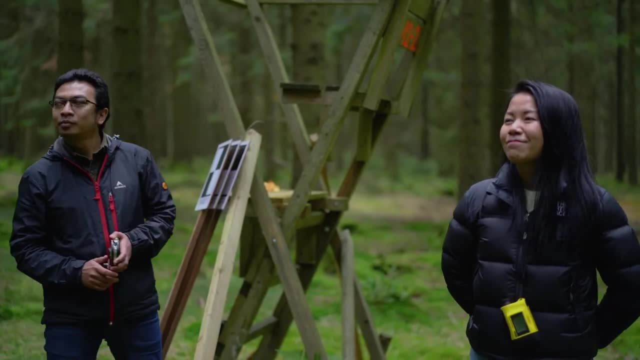 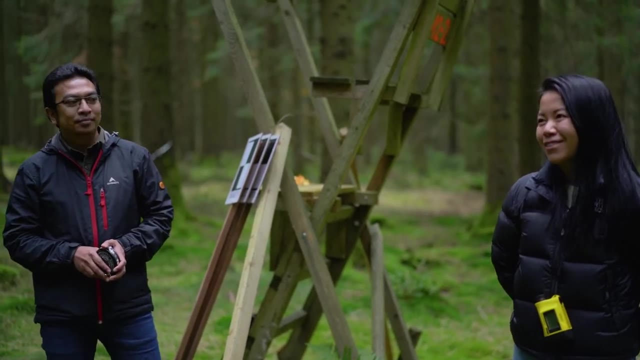 about a guess, Chu. what do you think? how much cubic meters in volume does such a spruce tree has? Around 4. So around 4 is a rough guess. Edwin, what is your opinion? Around 2, maybe, Maybe 2.. 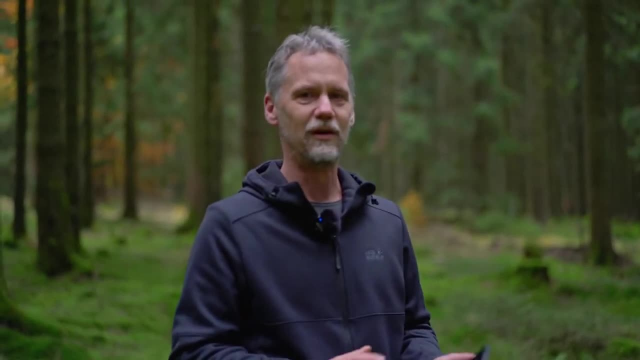 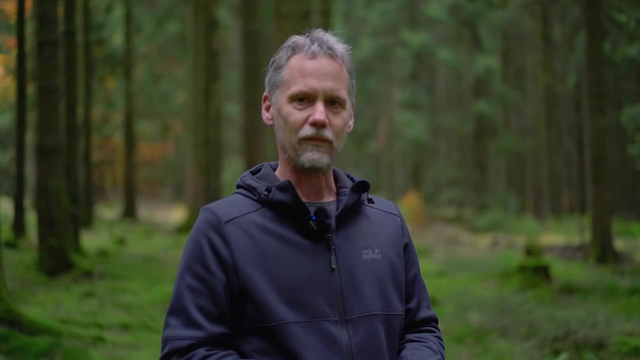 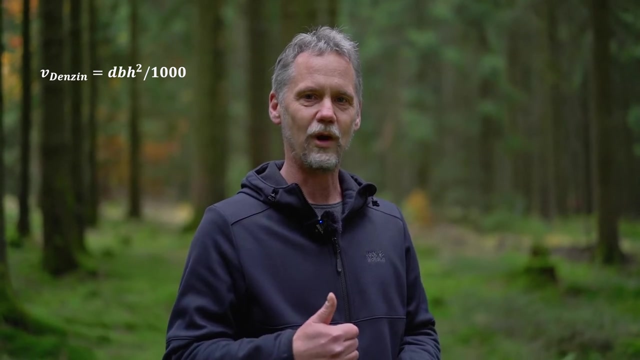 Or half of it. So somewhere between 2 and 4 is a rough estimate, but now we like to calculate it a little bit more accurate. So, as I told you before, the formula of Denzin is very simple. We take the diameter to the power of 2 and divide by 1000. And this formula doesn't make. 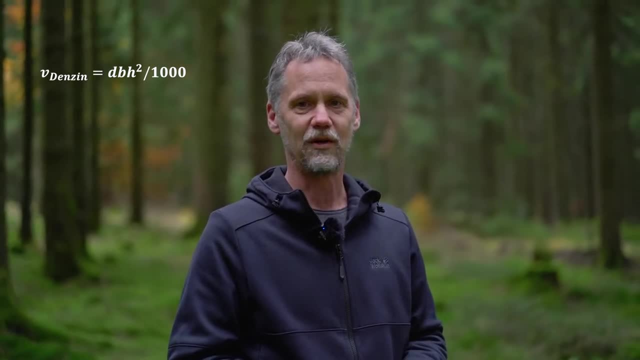 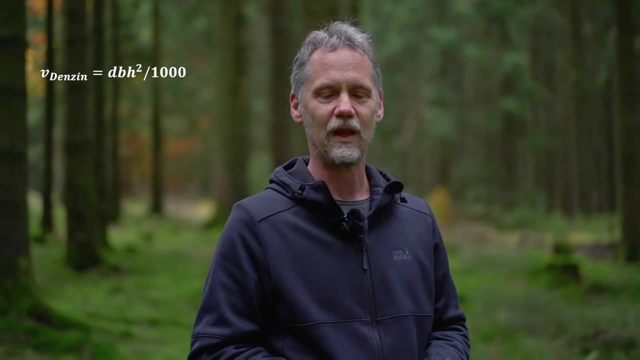 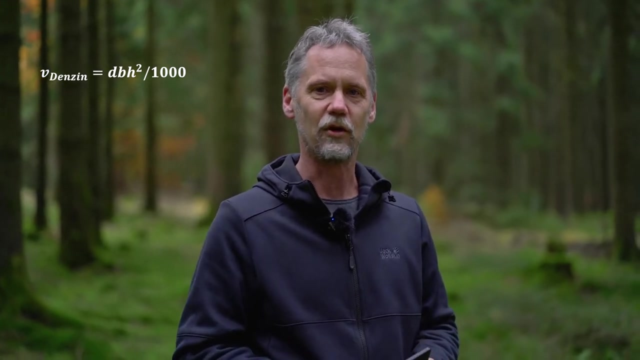 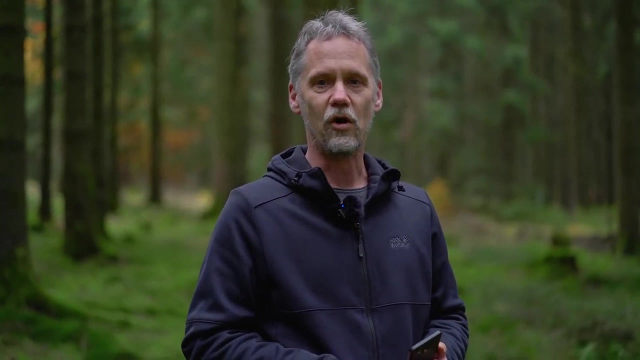 any sense from a mathematical perspective, because we are here entering the diameter in centimeters And we get a result in cubic meters. However, surprisingly, this formula works very well and Mr Denzin takes a lot of assumptions for this formula, For example, that the volume, the resulting volume, is for a norm height of 25 meters. 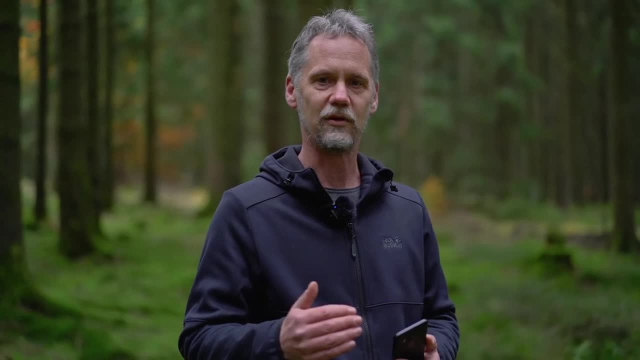 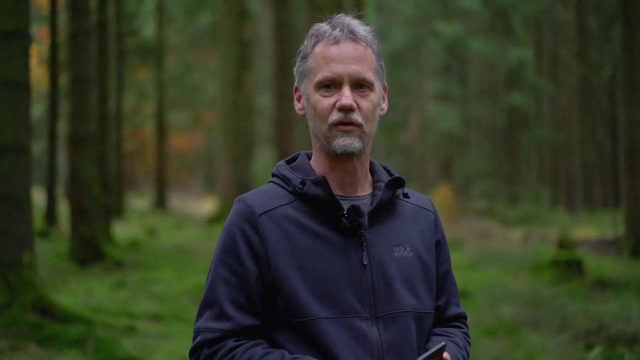 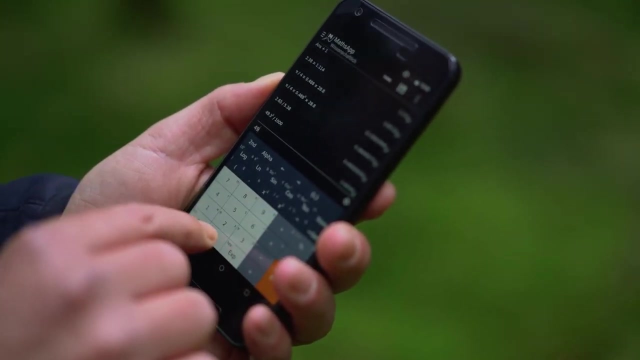 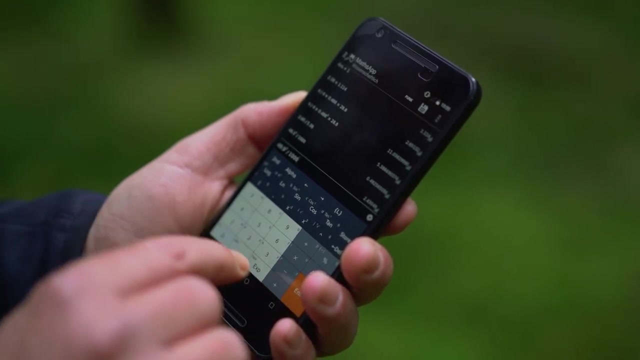 For each meter in height difference, negative or positive, we need to add or subtract 3% of the calculated volume as a correction factor. Ok, let's do the calculation. So we measured a diameter of 49.9.. We take this to the power of 2 and we divide this by 1000. And our result is 2.49 cubic meters. However, this is for a norm height of 25 meters. The actual height of this tree was 28.8 meters, So this is for a normal height of 25 meters. So let's calculate the difference: 28.8 minus 25.. 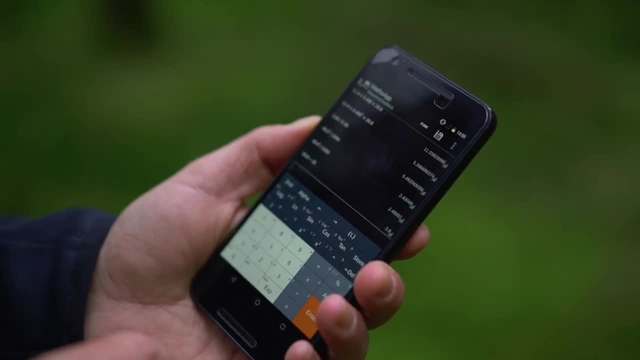 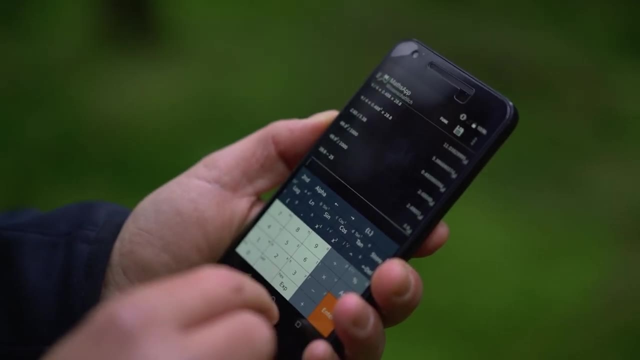 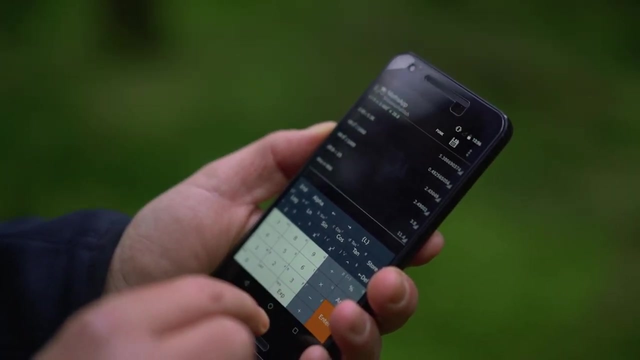 We have a difference of 3.8 meters And for each meter difference we need to add 3% to our first result. So we take this times 3%, 0.03.. So we need to add 11.4%. Ok, That means I need to calculate my first result, which was 2.49.. And I need to multiply with 1.114.. And the final result would be 2.77 cubic meters for this spruce tree. So 2.77 cubic meters is a rough estimate, but if you try out this formula, at least here: 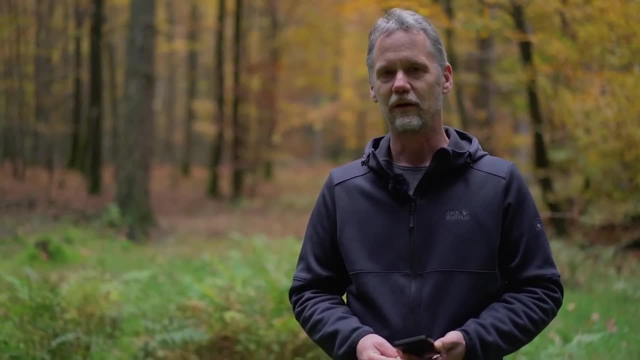 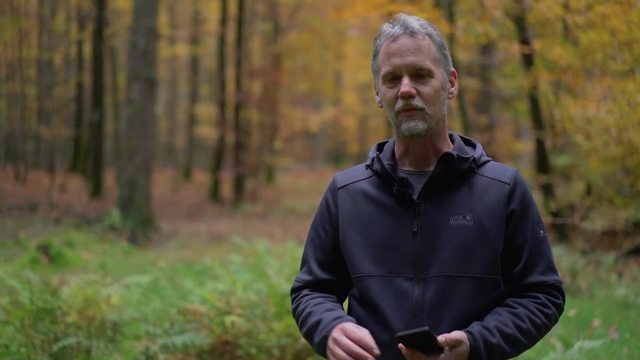 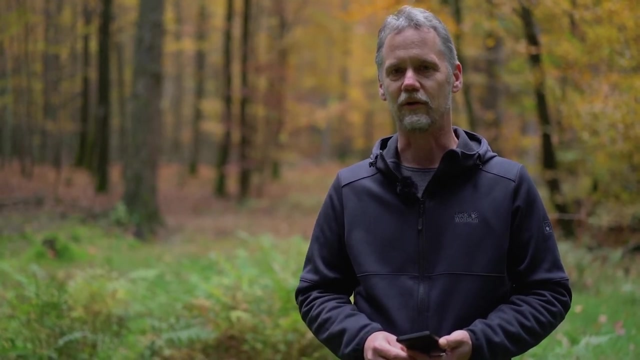 in Central Europe. in Germany it works quite well. Mr Densin also proposed better or more accurate correction factors for different tree species. But this norm height of 25 meters and the 3% plus minus is a general estimation formula. 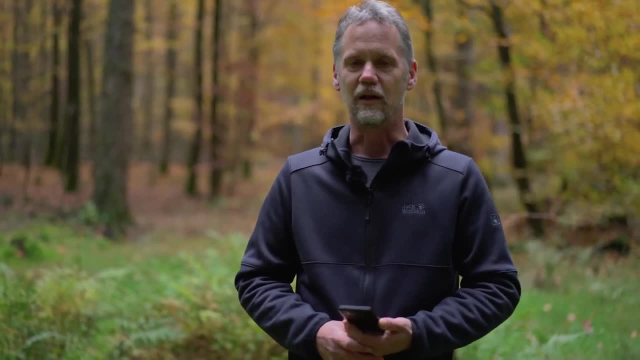 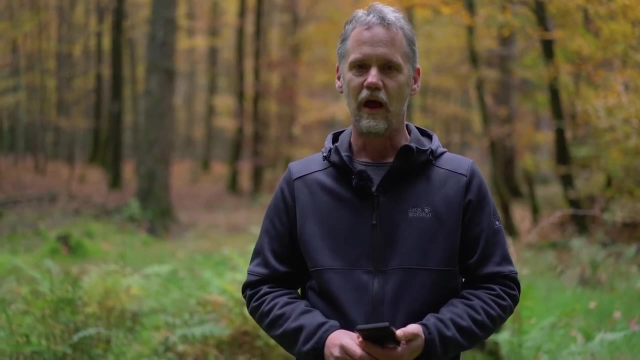 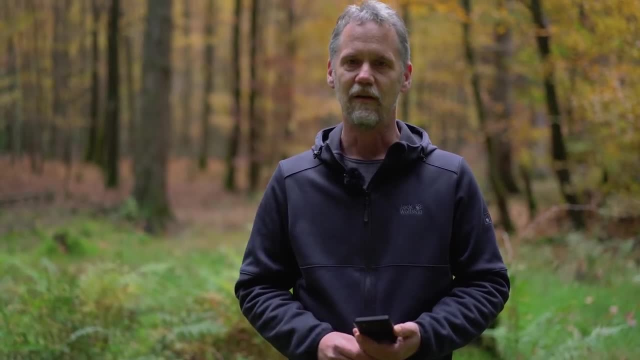 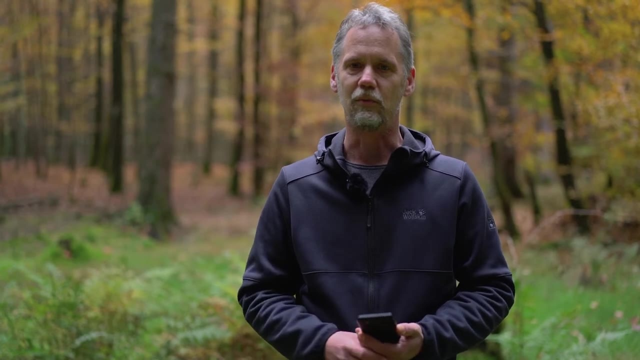 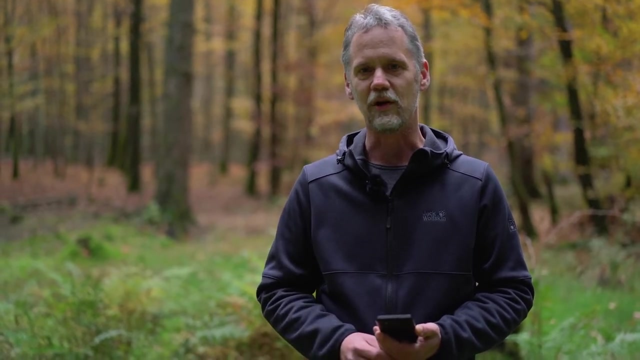 And we take the diameter, the dbh and the volume of the cylinder. And the length of the cylinder is the tree height. So it gives us the relation between this geometric shape of a cylinder and the actual wood volume inside the cylinder. If we now assume that the formula of Densin gives us a quite good approximation of the 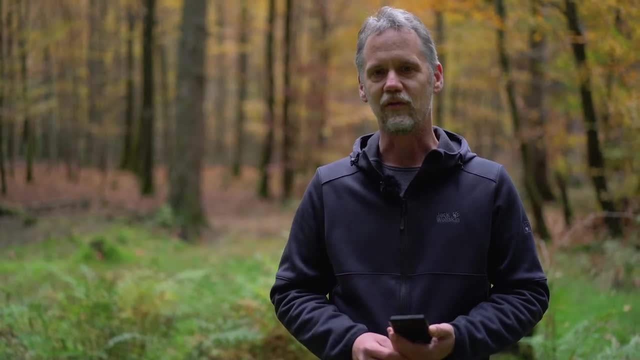 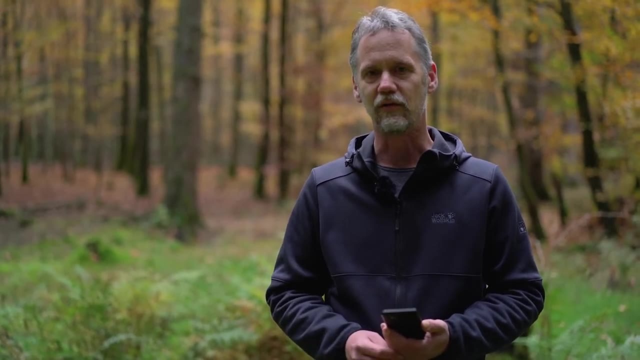 true volume. we can use this 2.77 cubic meters to calculate a form factor of this tree. What we need to do for this is we need to calculate the cylinder volume, taking the dbh we have measured and the tree height we have measured as input variables. Well, this is something that I 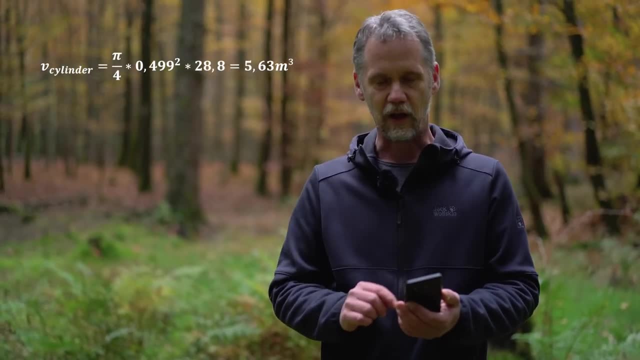 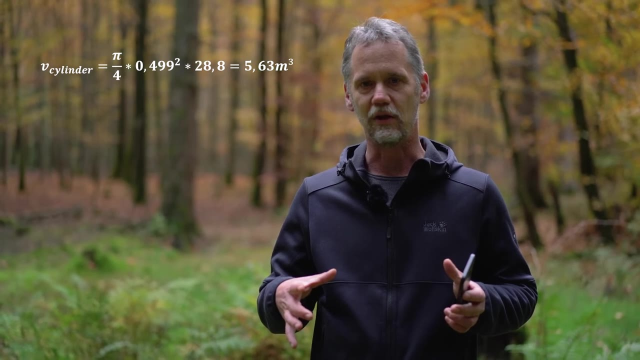 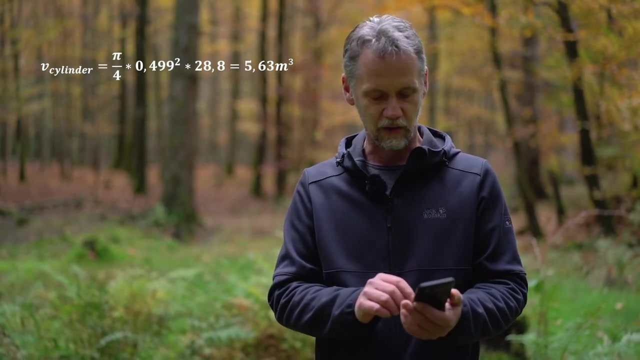 can do here for you. So we would need to calculate the basal area of the tree, the cross-sectional area, preferably in square meters, and we need to multiply this with the height of the tree To calculate the cross-sectional area of the single stem. I need to calculate p divided by 4. 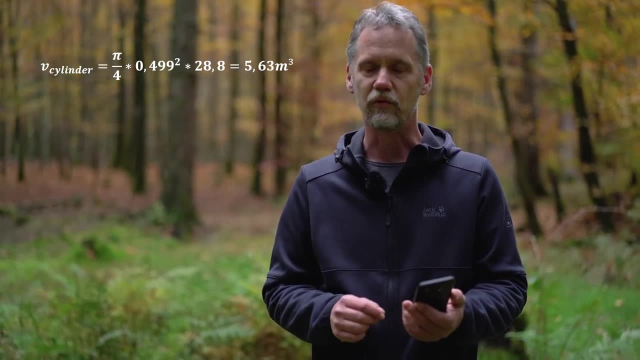 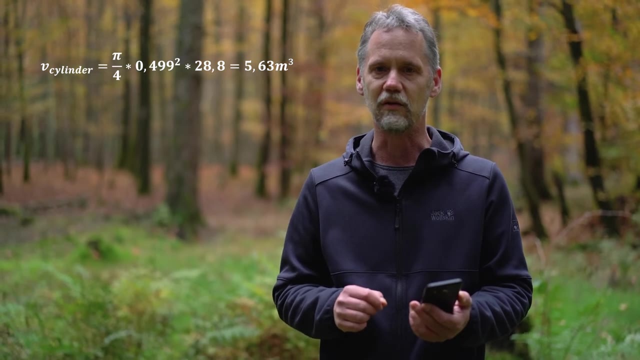 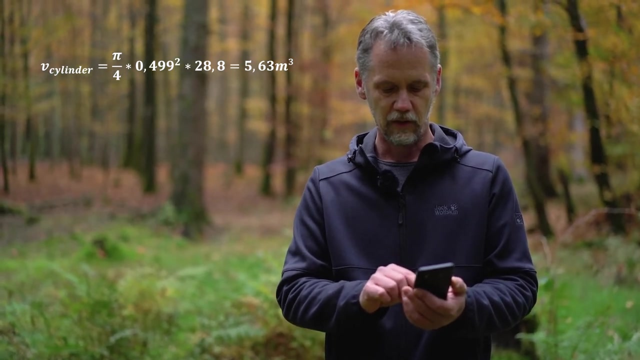 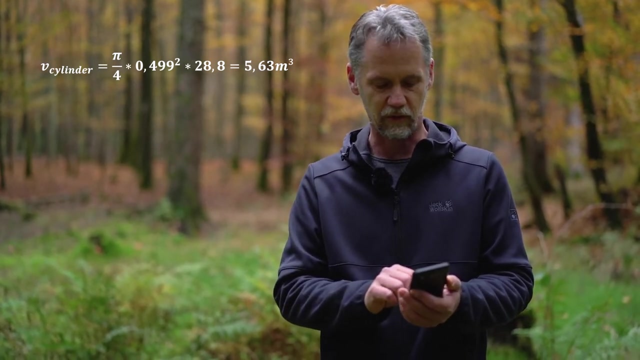 times the diameter to the power of 2.. Since I like to have it in cubic meters, at the end I direct directly input the diameter in meters. So it was 0.499 to the power of 2.. This is now our cross-sectional area, and now I multiply with the tree height of 28.8 meters.